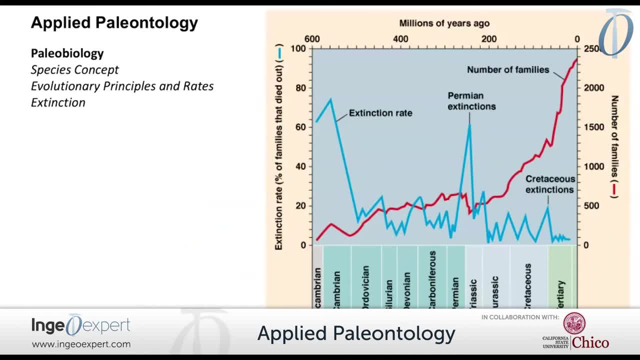 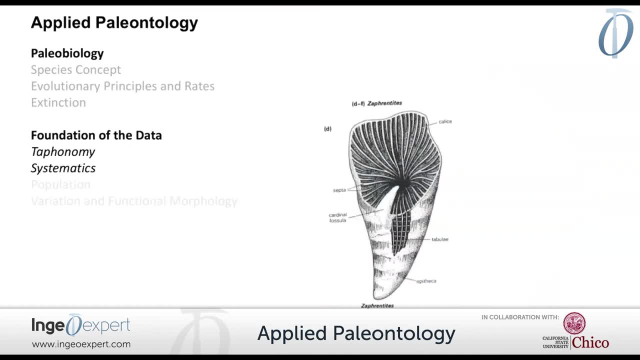 fossils to understand extinction. We then move into looking at the data that sells the fossils. We start with taphonomy- the making of a fossil move through systematics, or how we learn to name genus and species of fossils, and then look at how populations 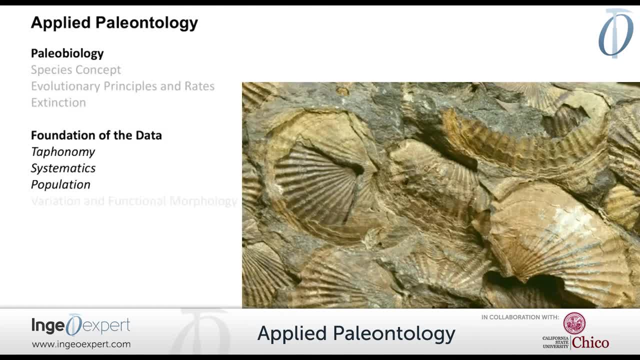 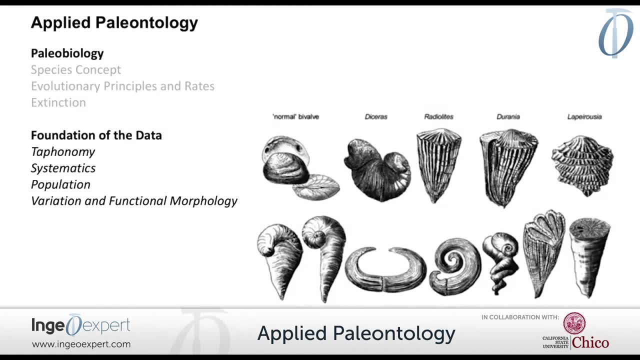 are recorded in the fossil record And ultimately, we'll talk about how we can use the data to develop with these unique shapes And particularly with these extinct organisms. we don't know about how the variation of their skeleton and their functional morphology might impact. 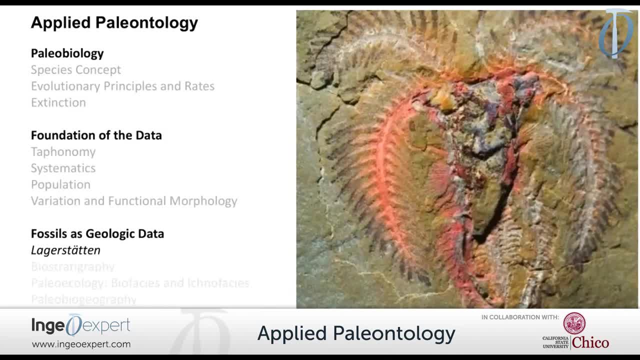 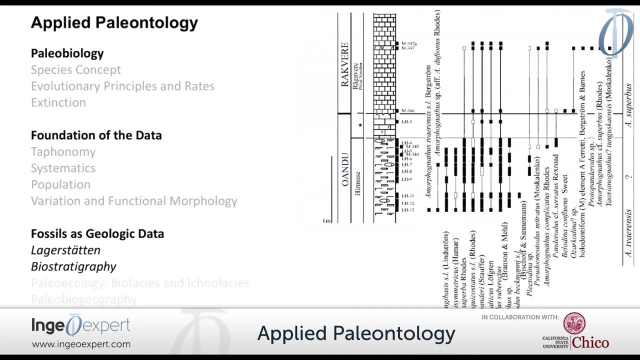 the way they got through life. The final part is actually using fossils as geologic data, And we'll start by looking at Loggerstetten, these amazing locations where fossils are really well preserved. We then move into the topic that most people associate with paleontology, that's biostratigraphy. 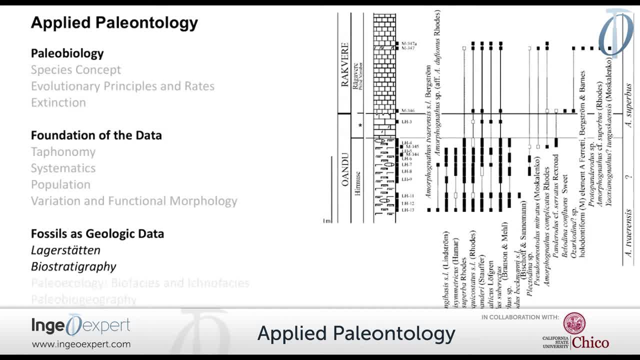 We're using fossils to age date rocks and corpse them. That is, we use fossil data to calculate the types of fossils which may or may not be well preserved, But we can also rocks and correlate rocks. From there we move into paleoecology. What can we learn looking at? 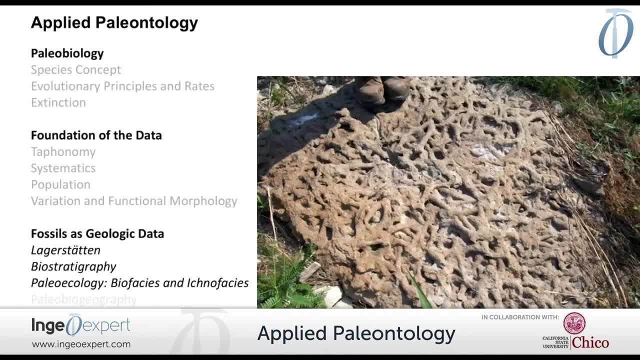 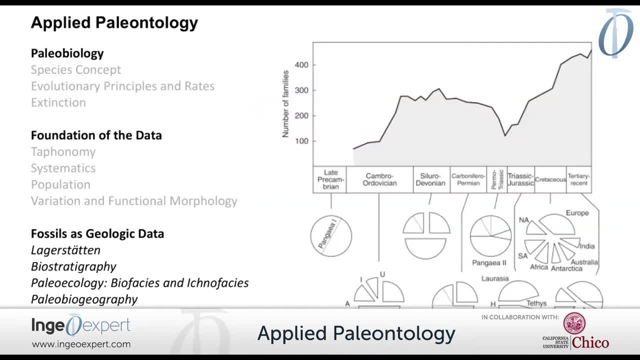 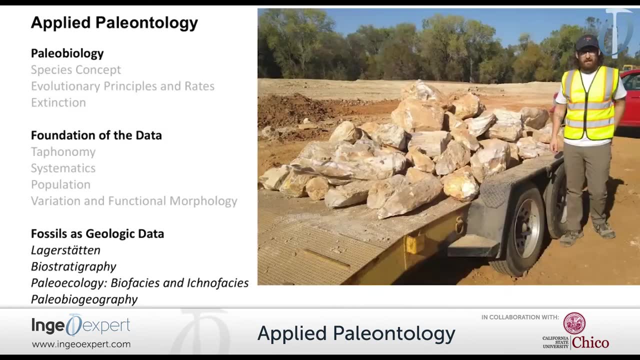 the behaviors or the distribution of organisms to understand how they interacted with themselves and their environment. We can then take fossils and look at a really big picture: paleobiogeography, or reconstructing continents and continental movements using fossils. And the final section. 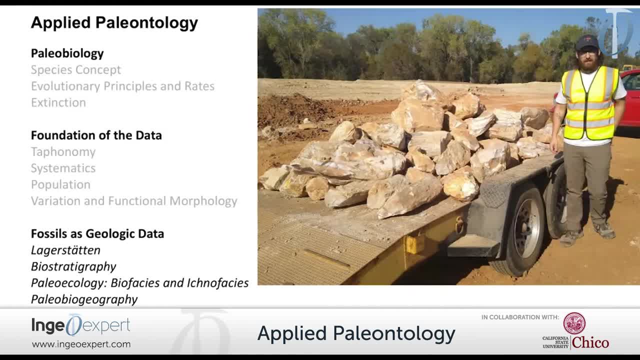 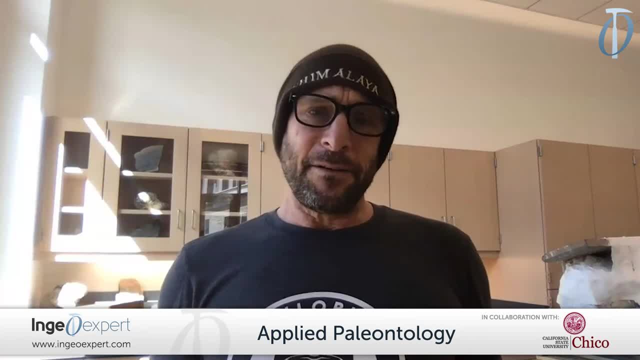 is regulation, laws and ethics which will vary around the world, but there are some similarities in how fossils are protected or how we might use fossils in an ethical manner. Now, at the beginning and end of each section, I'll host a live webinar introducing the new theme. 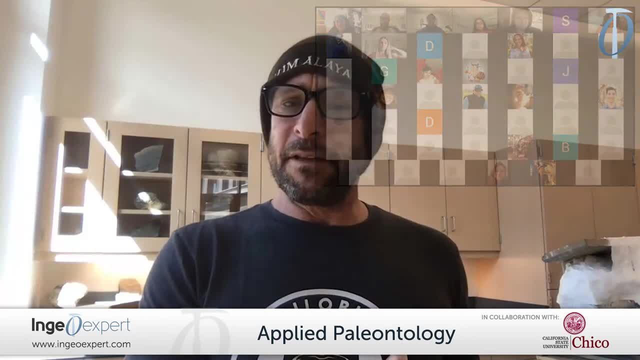 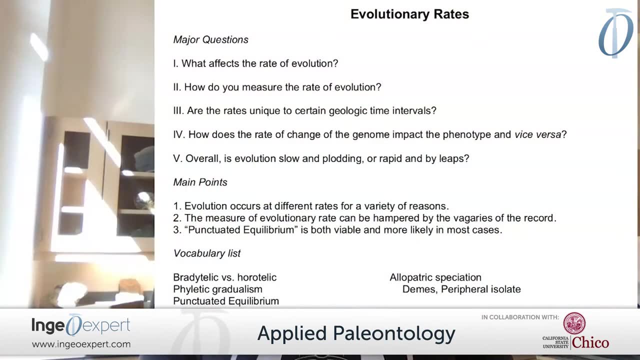 answering questions and then delving deeper into the topics of the preceding theme. for any questions you might have had, Instead of a textbook, I'm going to provide each of you with directed questions and vocabulary about each topic, with guidance on how to seek out the answers. 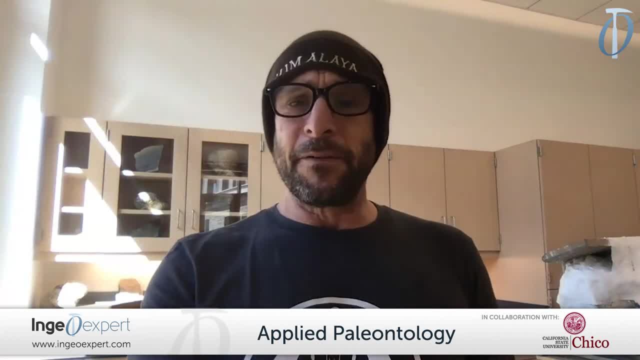 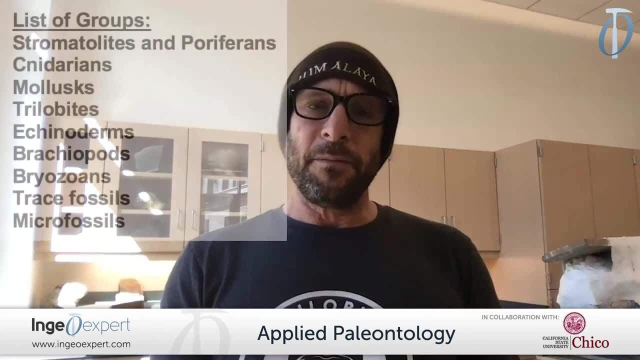 I'll also provide recorded lectures on the topic, and that might help clarify some issues. that isn't resolved from the beginning, But ultimately, this class is about fossils, and so, in parallel with themes, we will survey the major invertebrate groups you're likely to encounter, as well as trace fossils and microfossils.